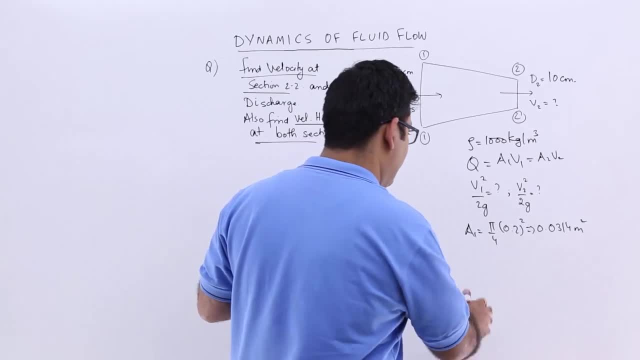 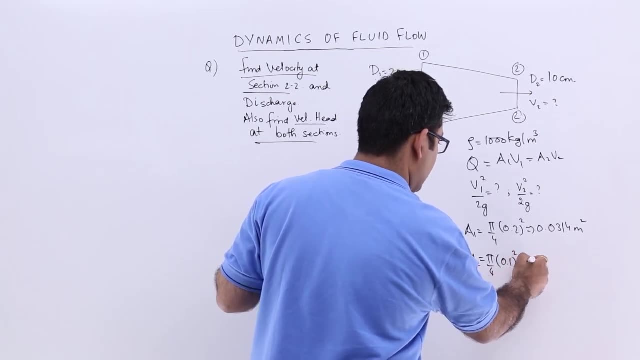 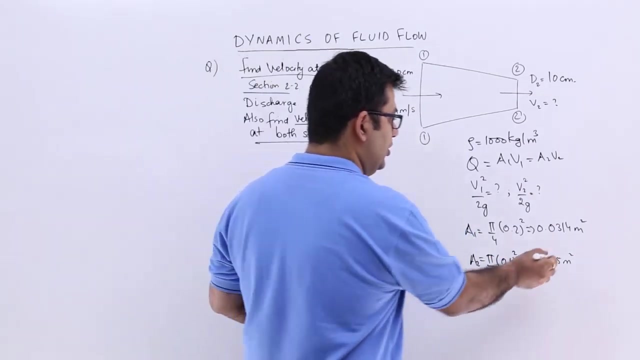 0.0314 meters square. Okay, Similarly, I can very well find out a2.. So a2 would be pi by 4 into 0.1 square, 0.00785 meter square. Okay, So I have two values of the two areas, Alright. 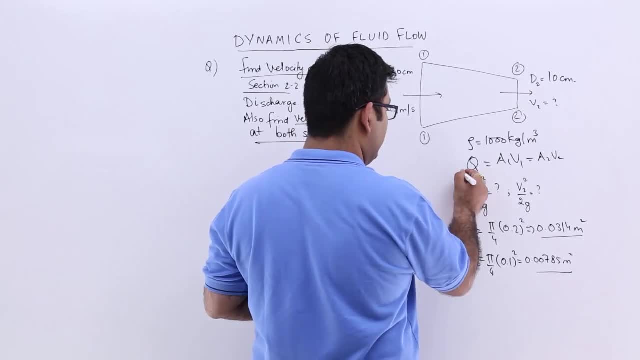 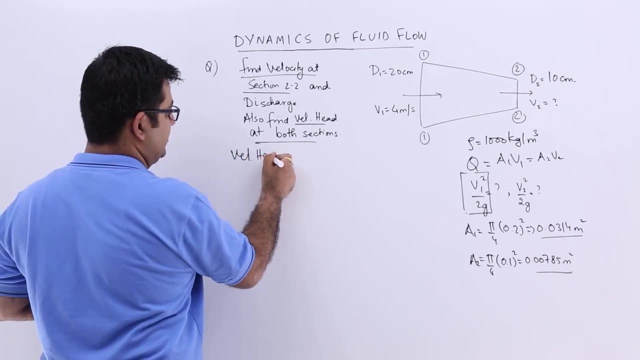 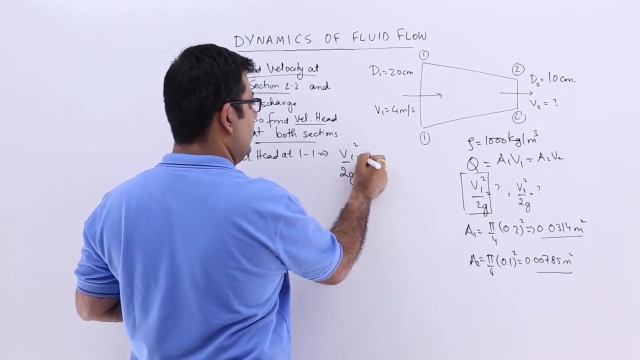 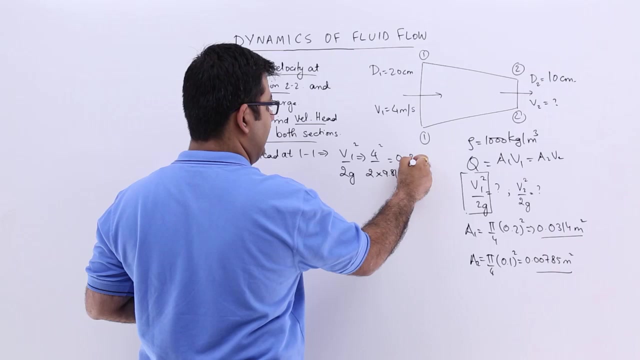 So I can let us start by finding out the velocity head at section 1.. So velocity head at section 1, that is 1,1.. This is equal to v1 square upon 2g. it will be equal to 4 square upon 2 into 9.81.. So this will be equal to 0.815 meters. So this is the velocity head. 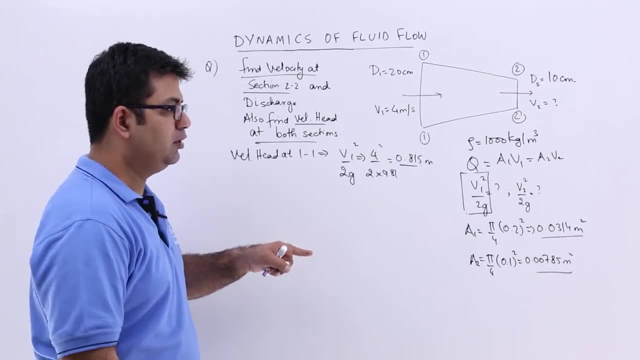 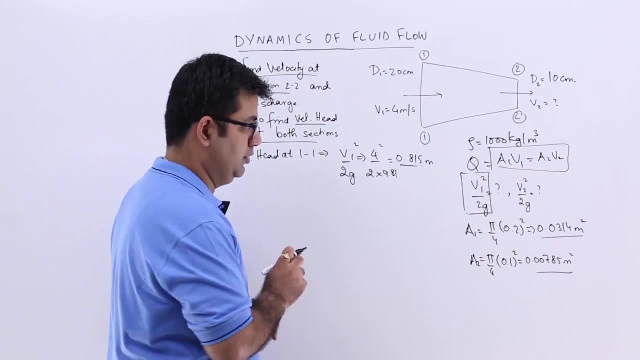 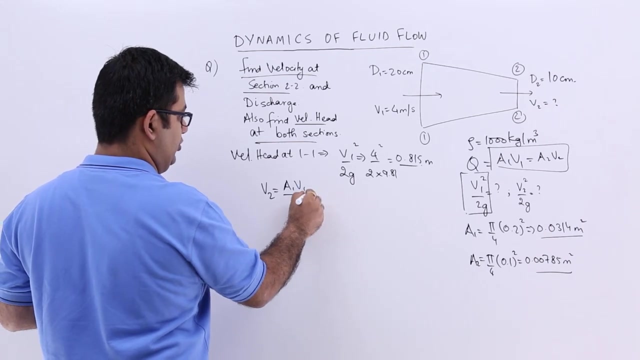 at section 1,1.. Now let us find out v2 first of all. So for v2 I need to apply this equation, which is known as the continuous velocity head, at section 1,1.. So this is the continuous continuity equation. So from that I can use: v2 is equal to a1 into v1 upon a2.. So a1 is: 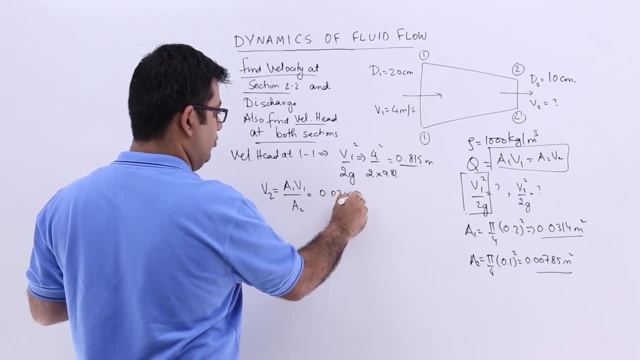 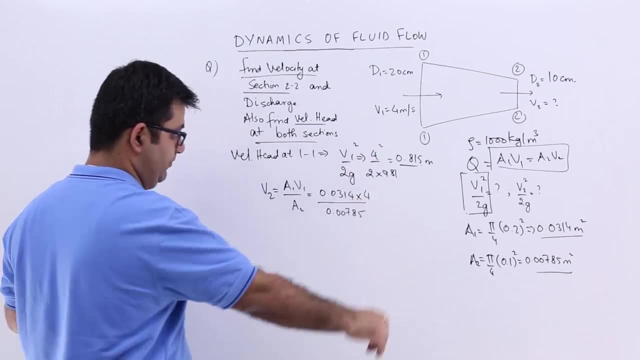 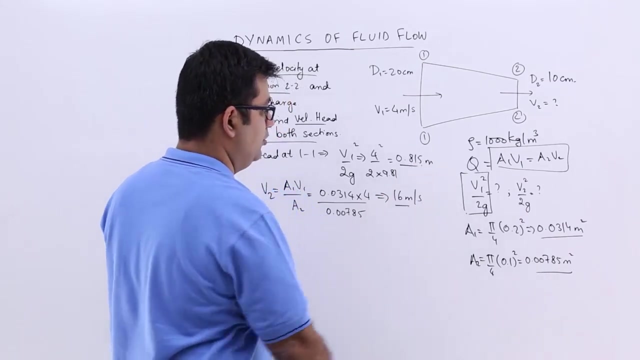 how much 0.0314 into 4 upon a2 is 0.00785.. So when you do the calculation with the help of your scientific calculators, you get the value of v2 as 16 meters per second. So this: 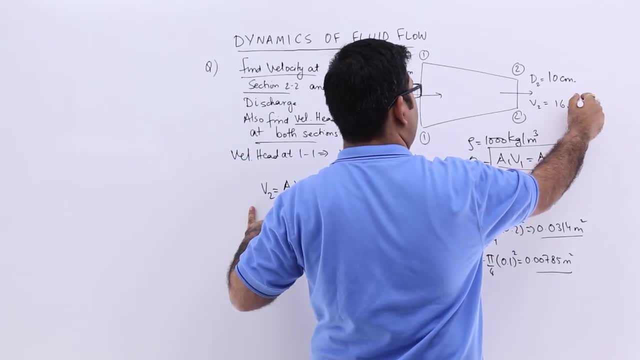 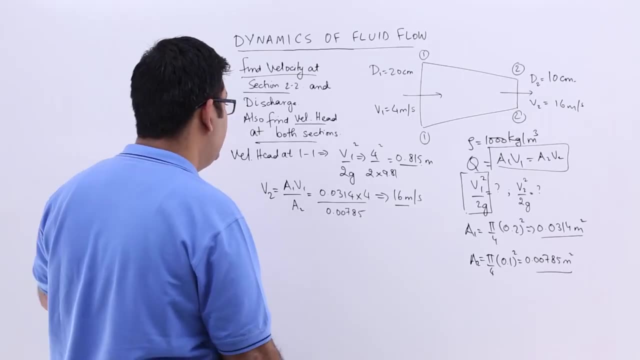 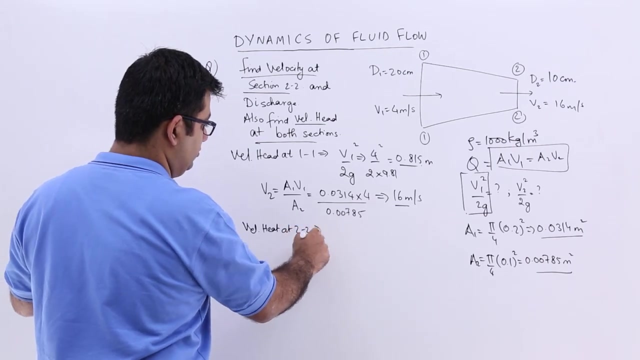 velocity head at section 1,1.. So this velocity head at section 1,1.. So this velocity head would be 16 meters per second. So with that velocity I can find out the velocity head also at section 2 and that would be velocity head at section 2,2.. This will be v2 square. 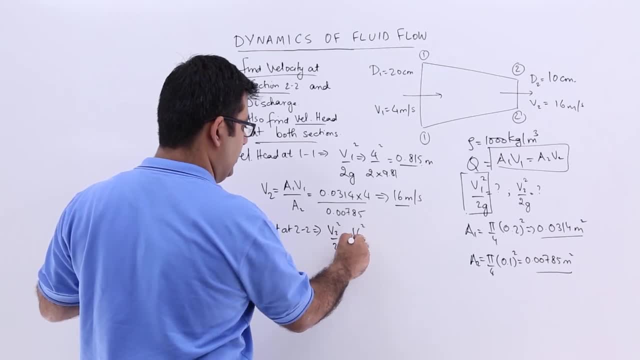 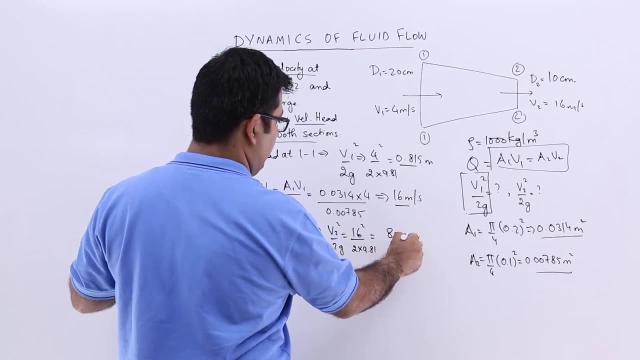 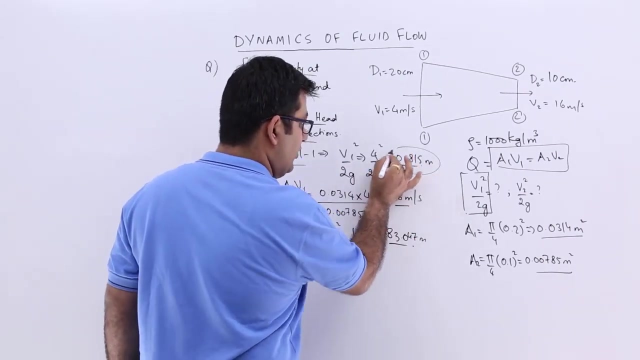 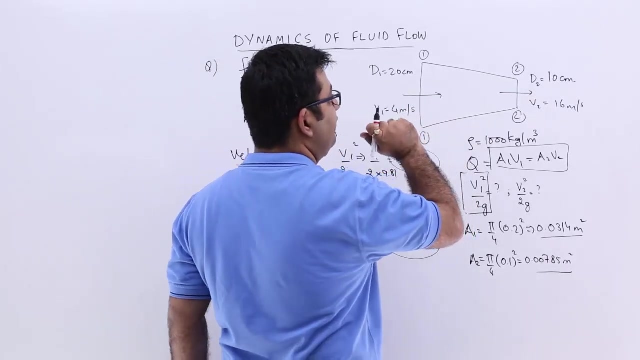 upon 2g, which means 16 square upon 2 into 9.81.. So that will be equal to 83.047 meters. So you can see that the velocity head at section 1 in comparison to the section 2.. So you know, this shows that in this kind of a section the velocity will increase at the. 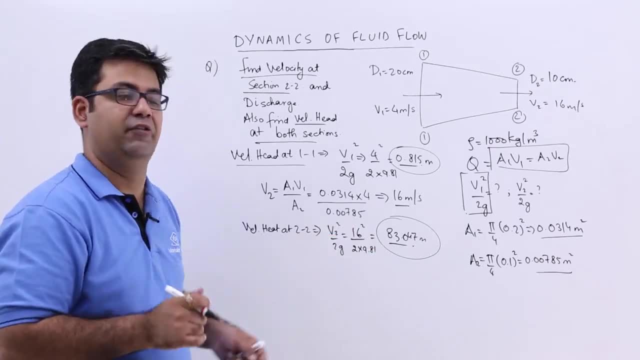 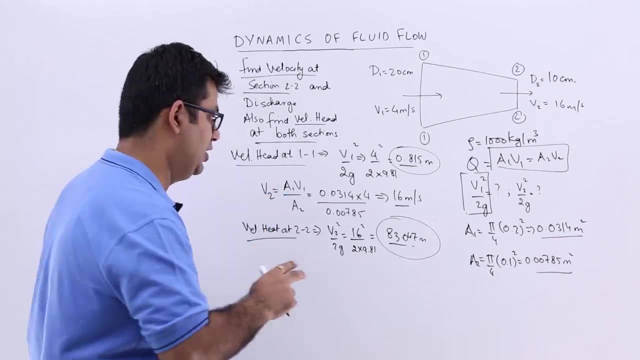 expense of pressure, because the total energy is conserved Right now. this is also done. The last part will be to find out the discharge. So discharge would be: q is equal to either we will use these two values or v1.. So this is the rate of discharge. So v1 is equal to.